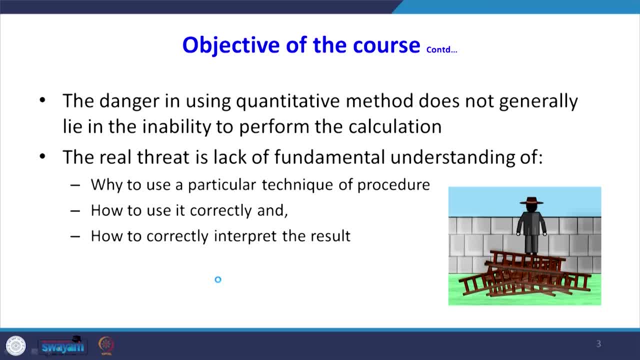 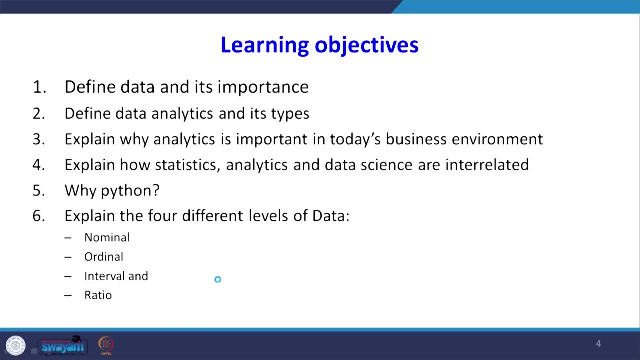 is lack of fundamental understanding of why to use particular technique or procedures and how to use it correctly and how to correctly interpret the result. This course will focus on how to choose the right technique. 1. So what was the learning objective of this class? That is, after completing this lecture? 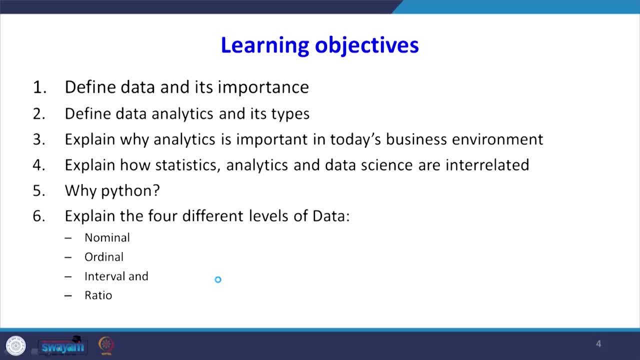 what you will learn. One is: you can define what is data and its importance. you can define what is data, analytics and types. you can explain why analytics is in today's business environment is so important. Then we can see how statistics, analytics and data science. 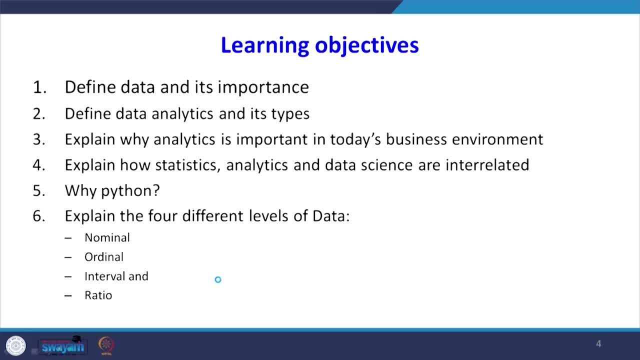 are integrated into the business environment are interrelated. there seems to be some overlap in this. we will clarify that. what is the difference, how these are overlapped, how these are interrelated, That in this course we are going to use a package called python- we will. I will explain. 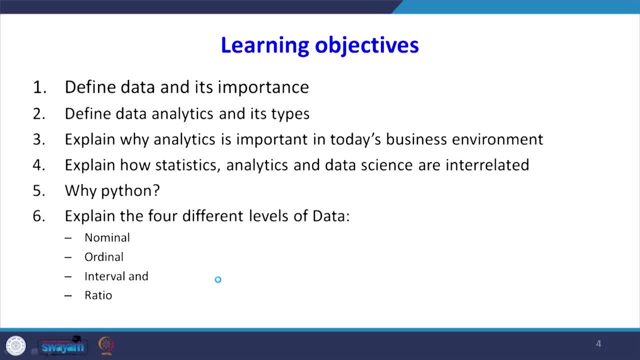 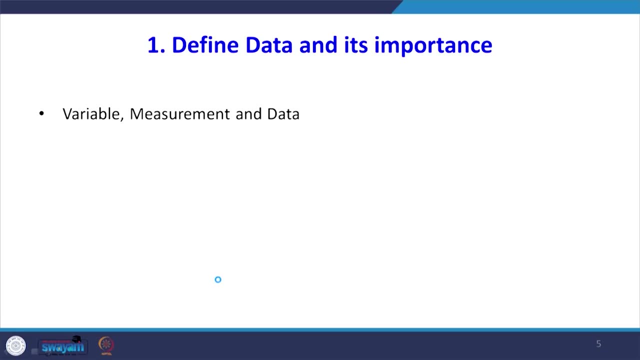 how, why it is important to use the python in this course. At the end of this session we will explain the four important levels of data, that is, nominal, ordinal, interval and ratio. Now we will go to the content. We will define data and importance. there are three term one is variable measurement and 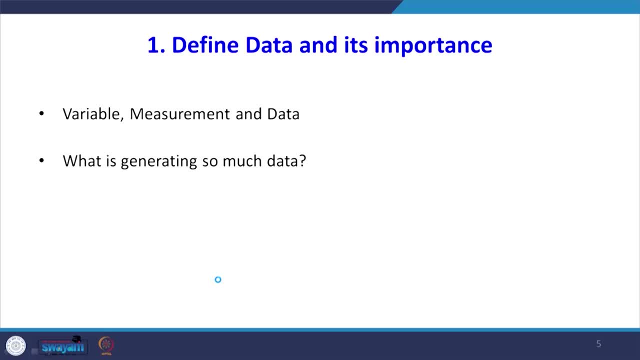 data. Next we will see what is generating so much data. next we will see how data add value to the business. then we will say why data is important. See the variables. measurement data- these are the terms which we are going to use frequently in this course. 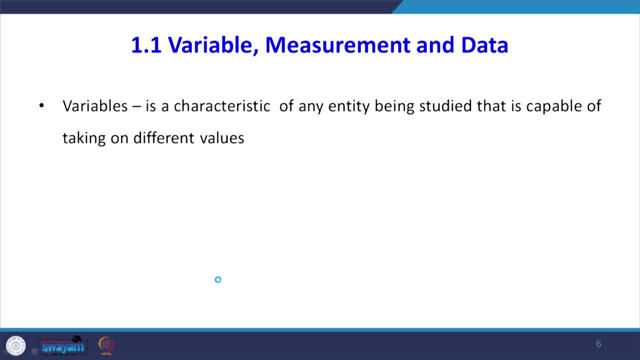 So what is a variable? Variable is a characteristics of any entity Being studied that is capable of taking on different values. Say, for example, x is the variable. it can take any values: it may be 1, it may be 2 or it may be 0, and so on. 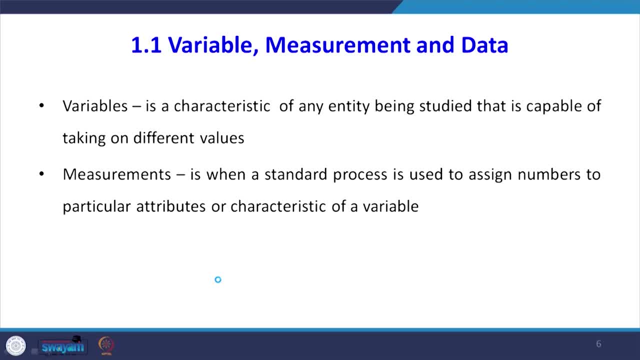 The measurement is when a standard process is used to assign numbers to a particular attributes or characteristics of variable is called a measurement. For that x. you want to substitute some values For that values you have to measure. You measure the characteristics of the variable. that is nothing but the your measurement. 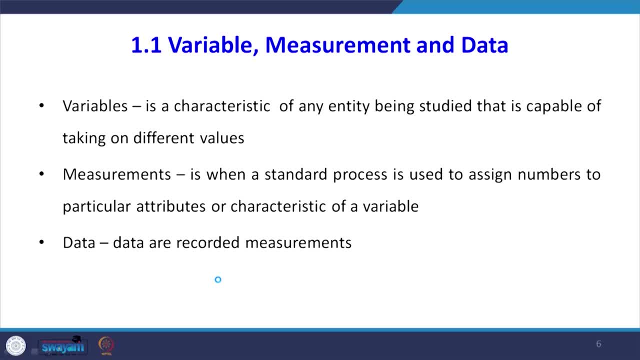 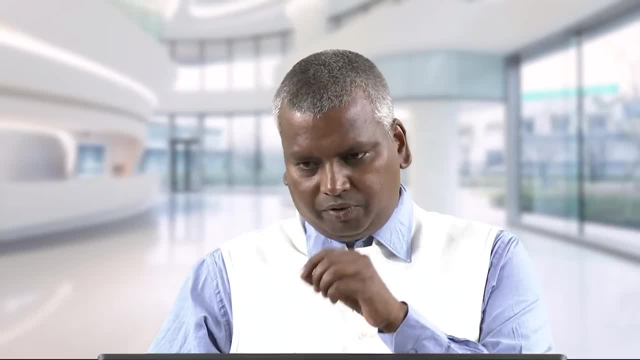 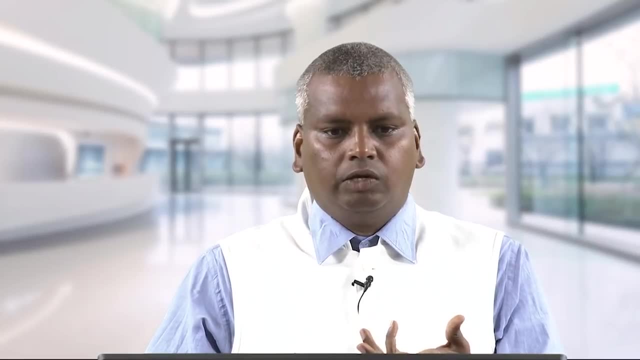 So then, what is the data? Data are recorded. measurement. So there is a variable. you measure the phenomena. after measuring that phenomena, you are substituting some value for the variable, so that the variable will take a particular value. that value is nothing but your data. 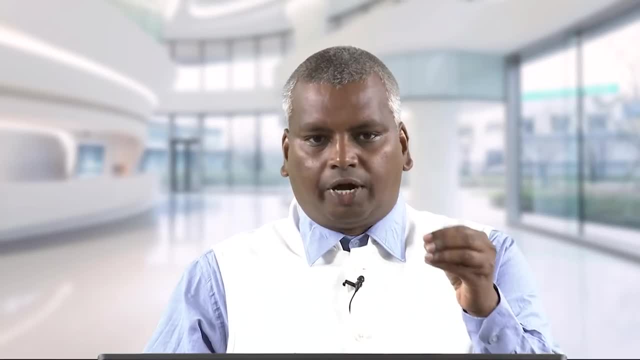 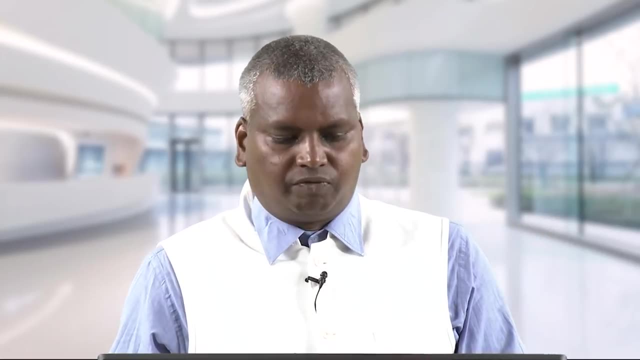 So x is the variable, For example. For example, number 5 is the data. How you are measuring that 5? That is called measurement. Then what is generating so much of data? Data can be generated different way: humans, machines, human-machines combined. 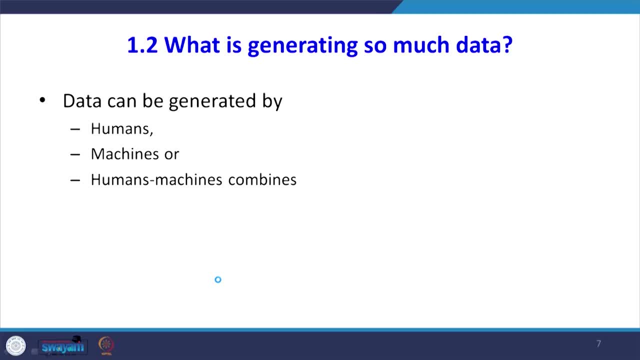 The humans-machines, human-machines combined in the sense now seen, everybody is having the various Facebook account, we have LinkedIn account, we are involved in various social network sites. Now, the availability data- Availability of the data is not the problem. ok. 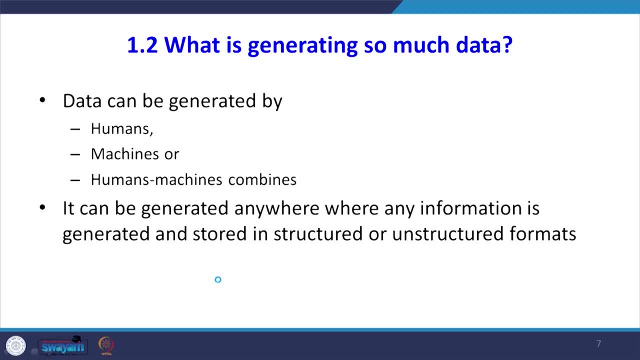 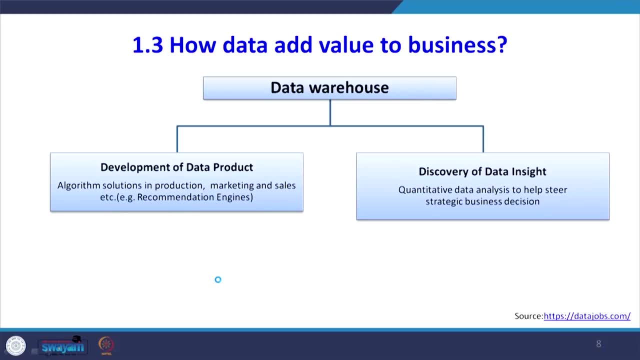 It can be generated anywhere where the information is generated and stored, and structured or unstructured format. So how the data add value to the business. So the data, after getting from various sources, assume that it is stored in the form of data warehouse. So the from the data warehouse, the data can be used for development of a data product. 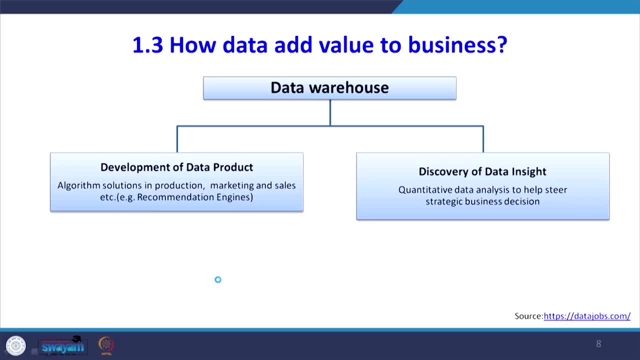 here we are using the word data product. In the coming slides I will explain exactly what is the data product. some examples: So the same data. if you look at the right hand side that can be used to get more insights from the data. ok, What do you mean by the data product? 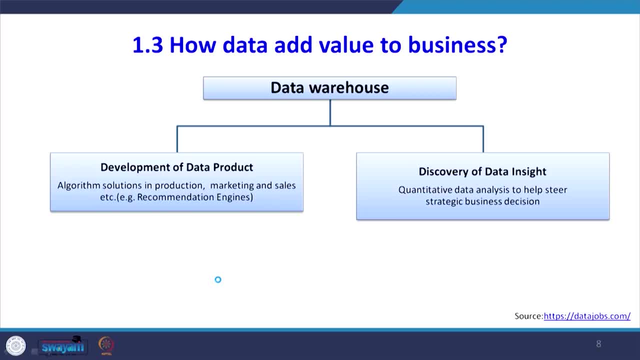 For example, algorithm solutions in production, marketing and sales. example of some data product: For example, recommendation engine. one of the example of example for data product: Suppose, if you go for Flipkart or Amazon, If you go for Amazon, If you are buying a particular product, that package, that software itself will recommend. 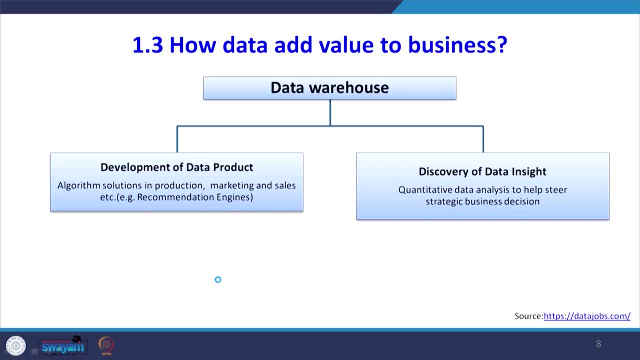 you what is the next product, possible product that you can buy? that is nothing but the recommendation engine. Even if you watch some YouTube videos on particular topic, that YouTube itself will suggest to you what are. the relevant videos are available, So that is a recommendation engine. that is one of the example of your data product. 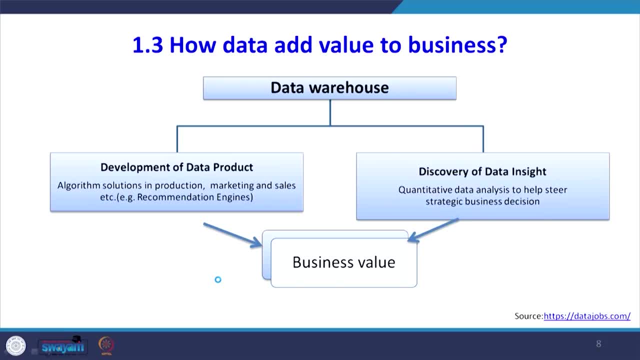 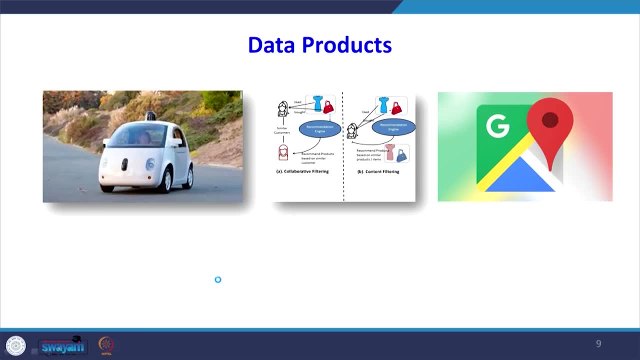 With the help of data, so that will help you to form a data product, or you can get a insight from the data that will add a business value to you. See, this is a example of your data products. this is the driverless car, Google car. 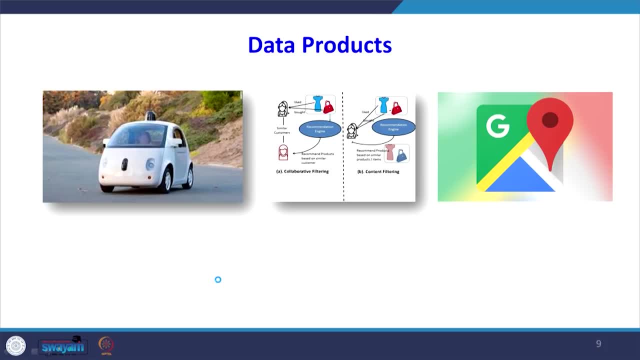 So the full concept of Google car is: with the help of data, it is detecting all other requirements for driving the cars. The next example is for recommendation engine. As I told you previously, when you buy any product, they will suggest you that, along with this product, the other product also can be purchased. 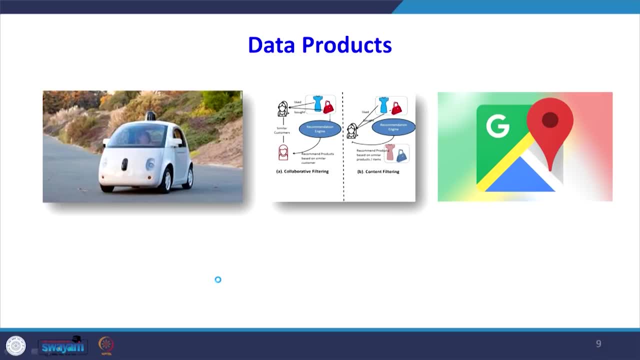 Another very common example for a data product is Google. The Google is a lot of applications there. one of the application of example for data product is a Google mapping. So the Google mapping is helping you to find out what is the right route, which route there. 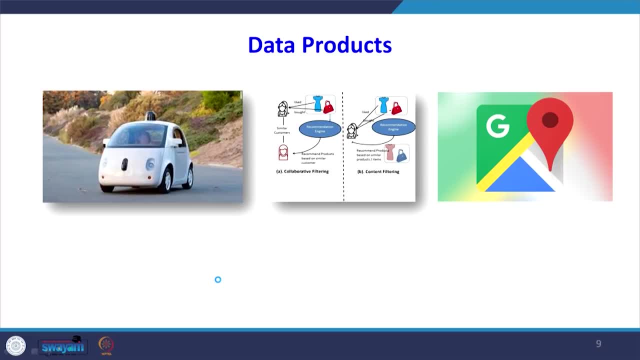 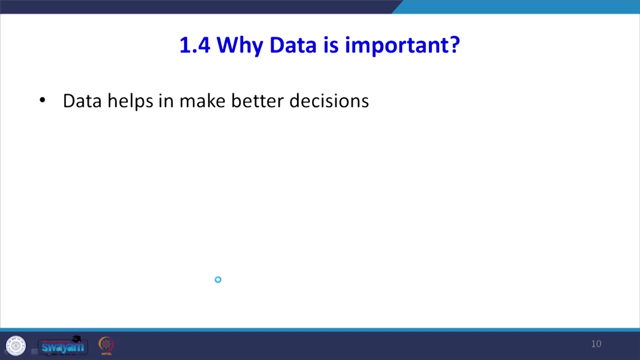 is a traffic and which route there is a toll booth. So this kind of information we can get it from the Google map. So this Google map is the one of example of your data production. Now why data is important. The data helps in making better decisions. data helps in solve problem by finding the 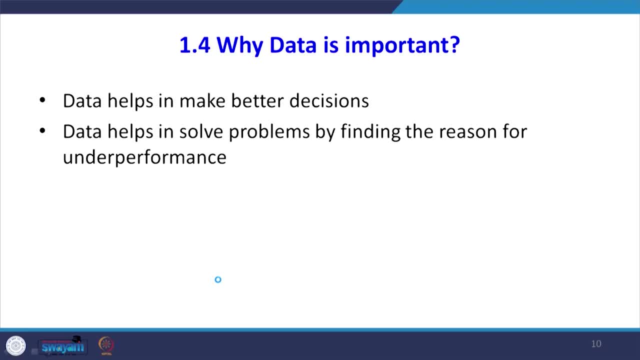 reason for under performance. Suppose some company it is not performing properly. by collecting the data, we can identify what was the reason for this. under performance: The data helps one to evaluate the performance. So what is the current performance? The data can also can be used. 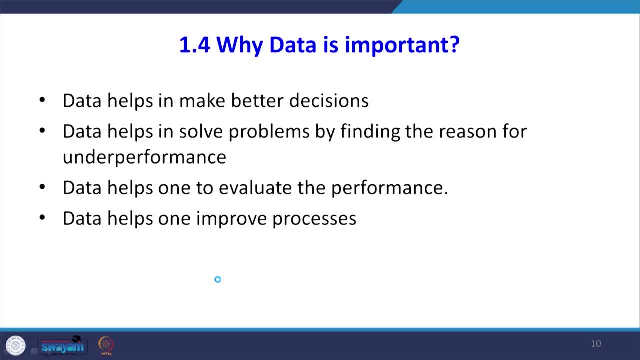 It can be used for benchmarking the performance of your business organization and after benchmarking data helps one improving the performance also. So data also can help to understand the consumers in the markets, especially in the marketing context. you can understand who are the right consumers and what kind of preferences they. 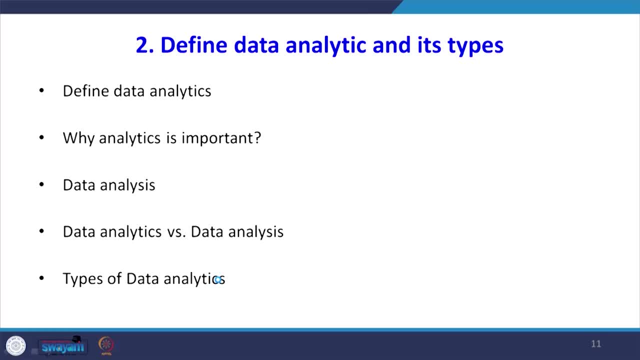 are having in the market. Next, we will define what is a data analytics and it is a types. So in this coming two, three slides we are going to discuss, we will define what is data analytics, then we say why analytics is important. then we will see the data analysis, then we 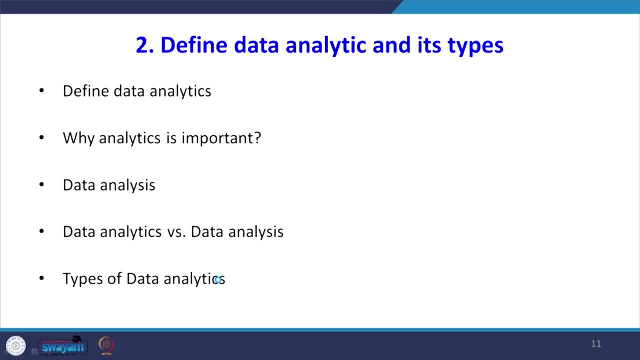 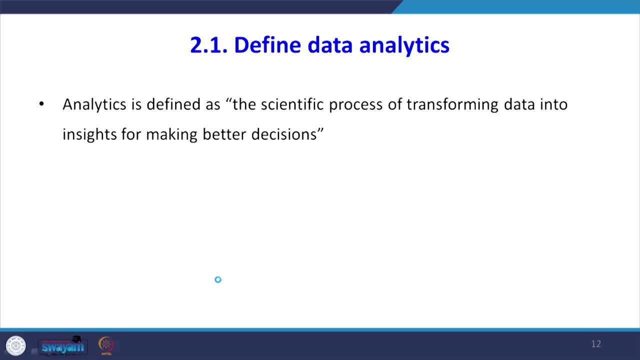 will see how data analytics is different from data analysis. at the end, we will see types of data analytics We will define. data analytics is the scientific process of transforming data into insights for making better decisions. See, it is an scientific process For transforming the data into for making better decisions. 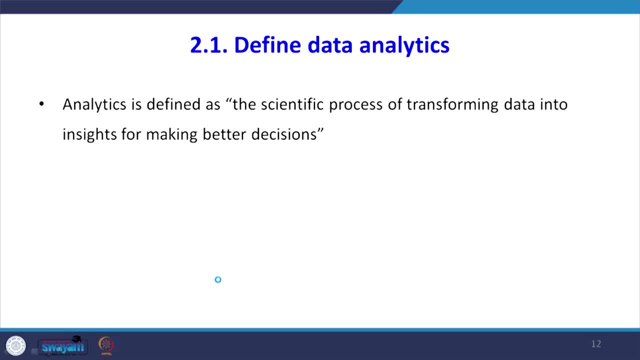 Even without data also, even without doing analytics also, you can make the decision, but it cannot, you cannot make the better decision without analytics. by the virtue of your experience and intuitions, you can take the decisions that also sometimes may be correct, but with the help of data, if you are making the decision, then that will enable you to make the better. 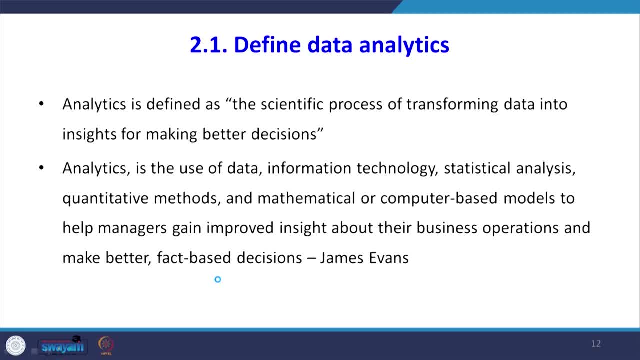 decisions. Next slide, please. Next slide. Next slide. This is James Evans. He has defined the data analytics in this way: It is the use of the data, information technology, statistical analysis, quantitative methods and mathematical or computer based models to help managers gain improved insight about. 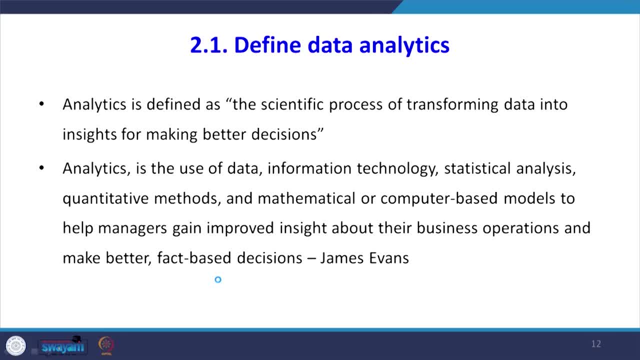 their business operations and make better fact based decisions. You see that there are many terms which are appearing here. one is IT, next one is a statistical analysis And next one is a quantitative methods, then mathematical knowledge and computer based models. So when we will see how these are interrelated in coming coming slides. 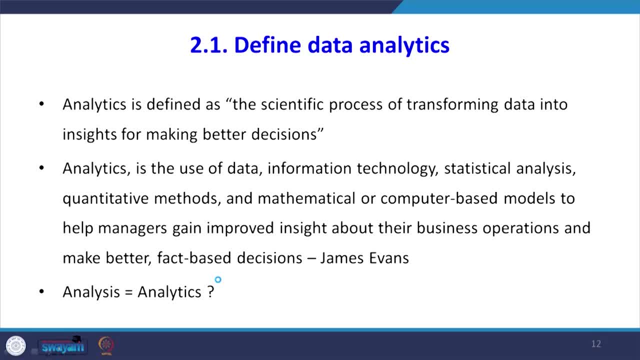 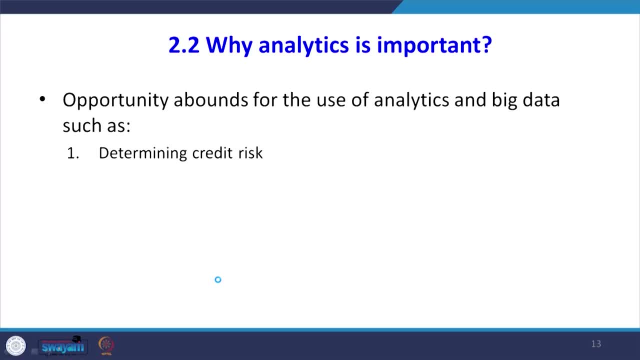 Generally, among the students, there is a confusion whether the analysis and analytics is same or different. Why analytics is important. The opportunity abounds for the use of analytics and big data, such as for determining the credit risk for developing new medicines, especially in healthcare. the healthcare analytics is 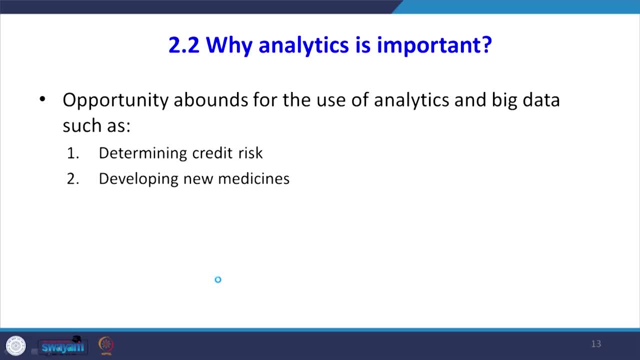 an emerging that is helping you to identify what is the correct medicines, Finding more efficient ways to deliver product and services and, for example, in the banking context. data analytics is used for preventing the fraud and it is uncovering the cyber threats. with the help of data analytics, you can find out the possible cyber crimes and 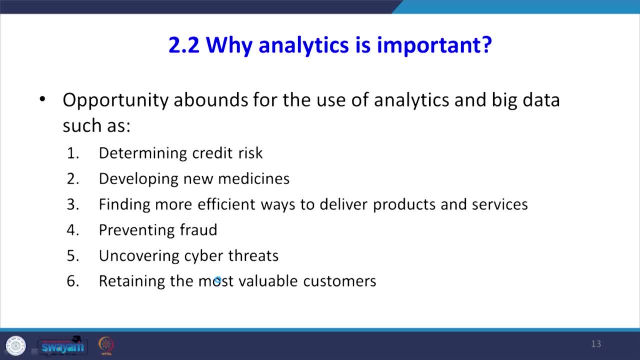 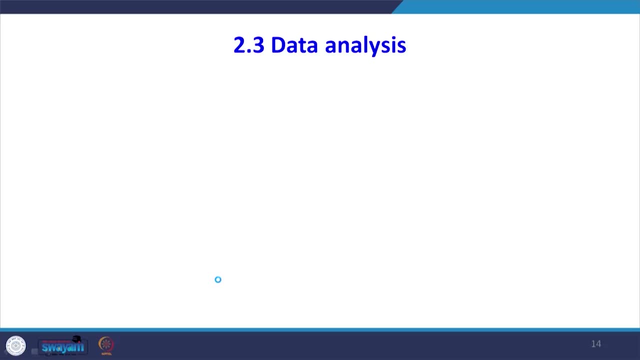 we can detect it, we can prevent it, And data analytics also important for retaining the most valuable customers. We can identify who is your valuable customer or non valuable customers, So we can focus on more on our valuable customers. ok, Now, what is the data? analysis is the process of examining, transforming and arranging the 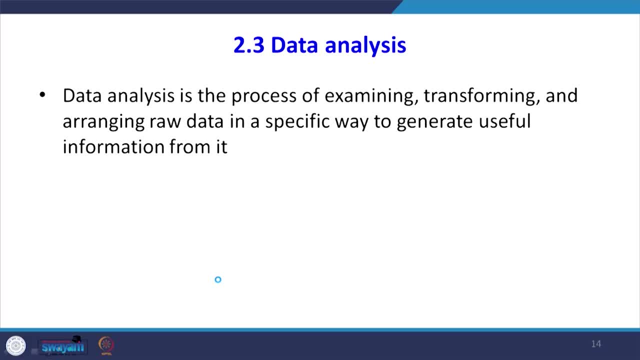 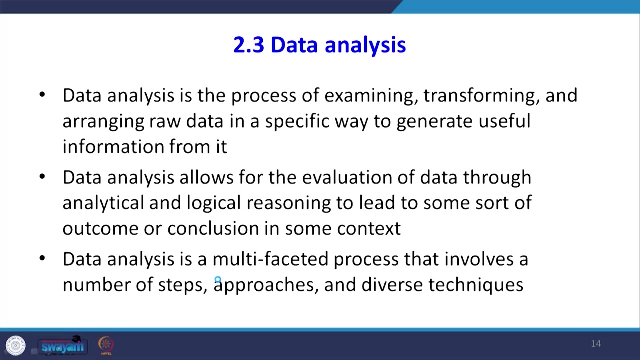 data, managing raw data in a specific way to generate useful, useful information from it. So data analysis allows for the evaluation of data through analytical and logical reasoning to lead to some sort of outcome or conclusion. in some context, Data analysis is a multifaceted process that involves a number of steps, approaches and 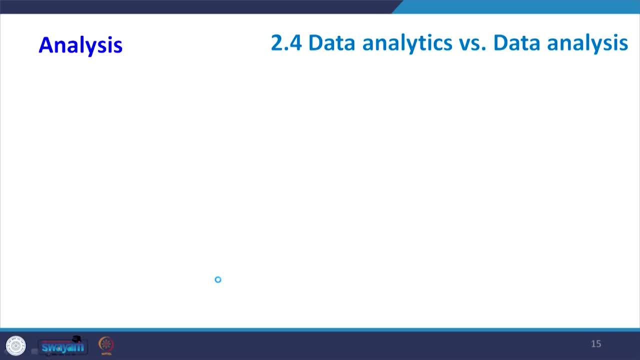 diverse techniques that we will see in coming lecture. So now we will see what is the analysis. is data analysis and data analytics? When you say analysis is when you say data analysis, it is something about what has happened in the past, So we will explain why that has happened. we will explain how it has happened. yeah, 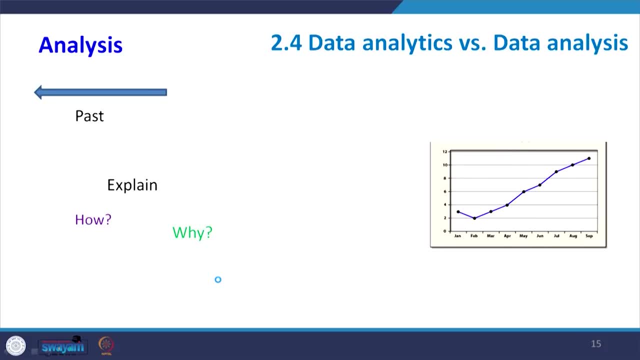 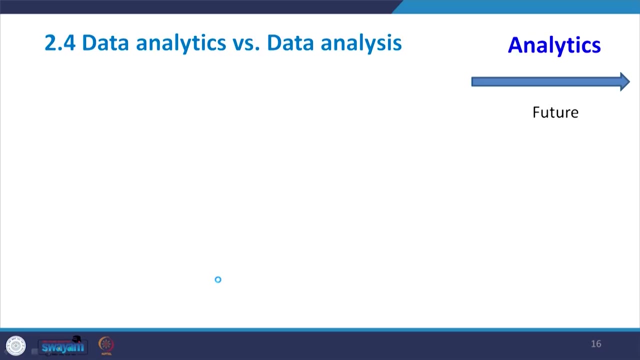 we can explain why it has happened. For example, when we say data analysis, that is nothing about studying about what has happened. it is like kind of a post-mortem analysis. what has happened in the past, ok, Ok. In the contrary, the analytics is studying about what will happen in future and with 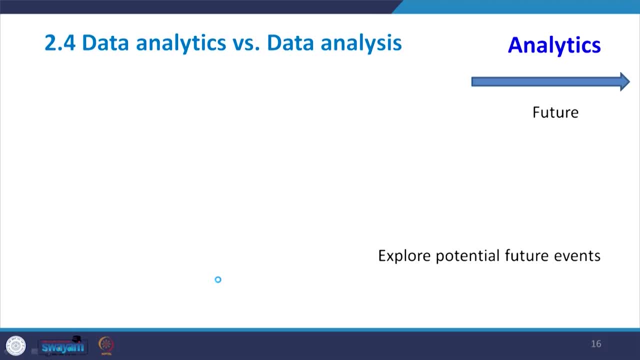 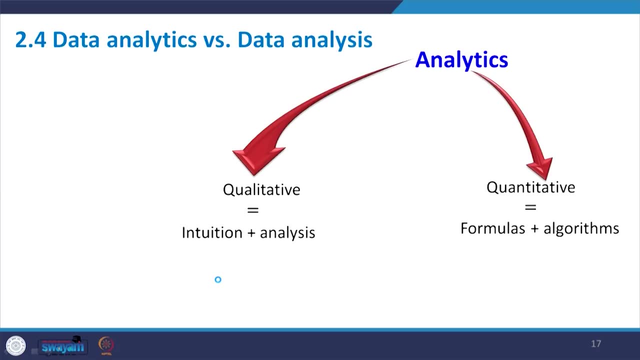 the help of analytics we can predict, explore possible potential future events. So the analytics is maybe qualitative or quantitative, for example in analytics. if we say qualitative analytics, so it is the decision mostly based on the intuition. But when you say in quantitative, where with the help of formulas, with the help of algorithms, 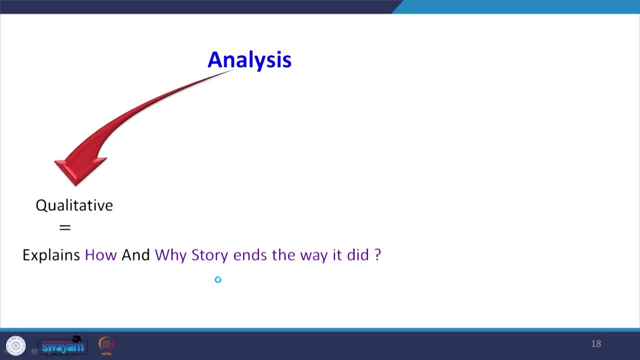 we will make the decisions. So in the analysis- data analysis also- we can go for qualitative. we can explain how and why a story ends in that way it did. When we say in quantitative, we can say how the sales decreased in the last summer. 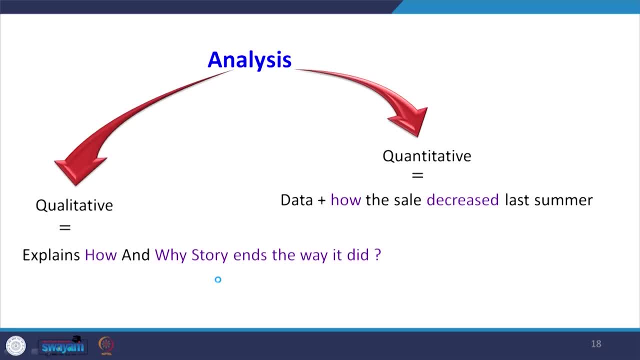 Say, when I say, as I am repeating, when you say analysis is something studying about what has happened in the past, ok, Ok. So it is not exactly analysis equal to analytics. Similarly, when you say data analysis is different, data analytics is different, similarly business. 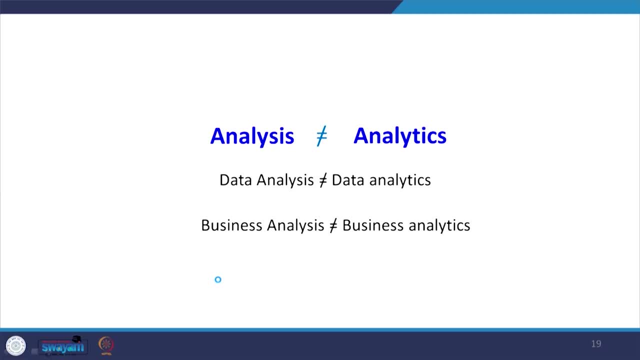 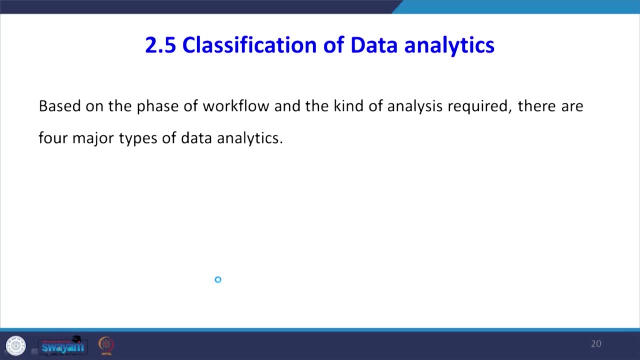 analysis is different. business analytics, When you say, analytics is nothing but studying about the future events with the help of the past data. Next, we will go for classification of data analytics Based on the phase of workflow and kind of analysis required. Ok, 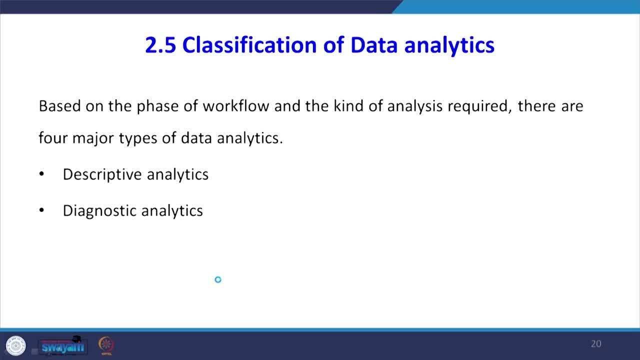 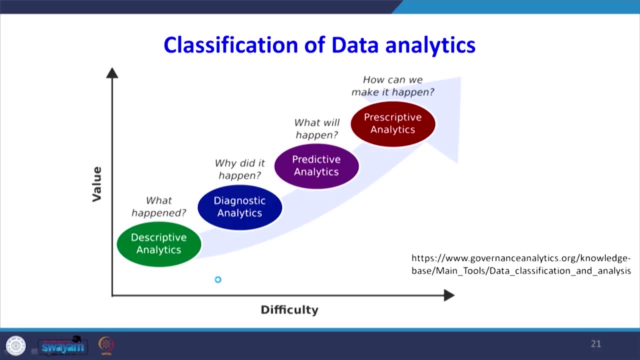 There are 4 major types of data analytics. one is descriptive analytics, diagnostic analytics, predictive analytics and prescriptive analytics. We will see these 4 types of analytics in detail in coming classes. If we look at the difficulty and the kind of value which we can get from different types, 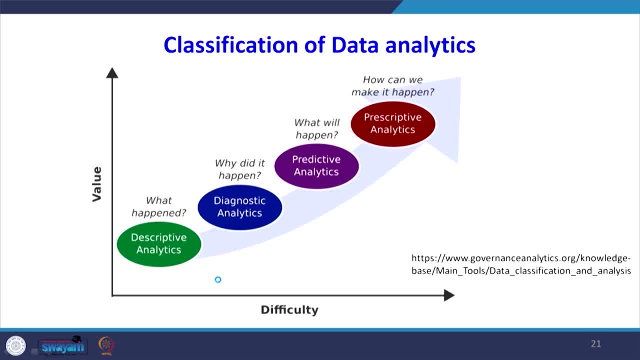 of analytics. this picture shows, for example, when you see the descriptive analytics that will answer what happened. Diagnostic analytics will help you to answer: why did it happen? Predictive analytics will help you what will happen. Prescriptive analytics will help you to answer: how can we make it happen? 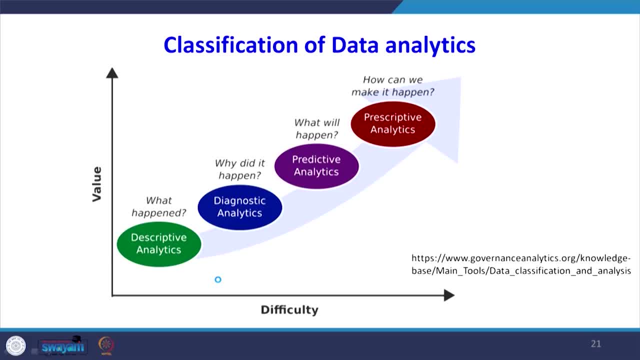 That is one context. When you look at the level of difficulty, you see that the descriptive analytics is level of difficulty is very less, and the contrary. when you look at the prescriptive analytics, the difficulty less. Ok, Ok, The level is more and the value also value in the sense, business value, with which adds. 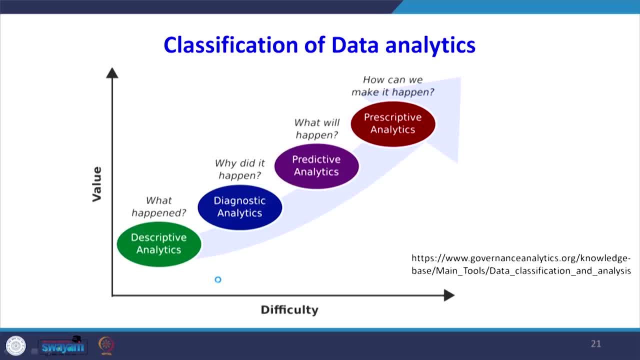 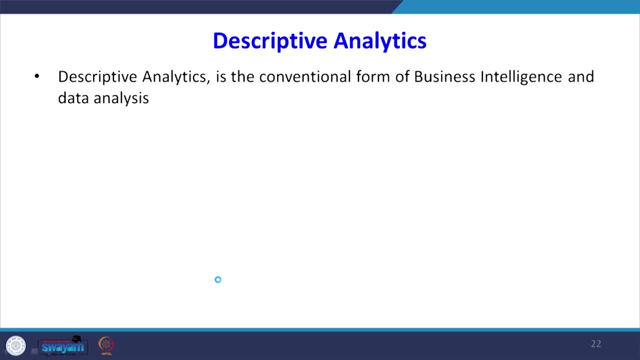 to you also more So when there is a more difficulty, there is a more value. Ok, Then we will see what is the descriptive analytics. Descriptive analytics is the conventional form of business intelligence or data analysis. It seeks to provide a depiction or summary view of facts and figures. 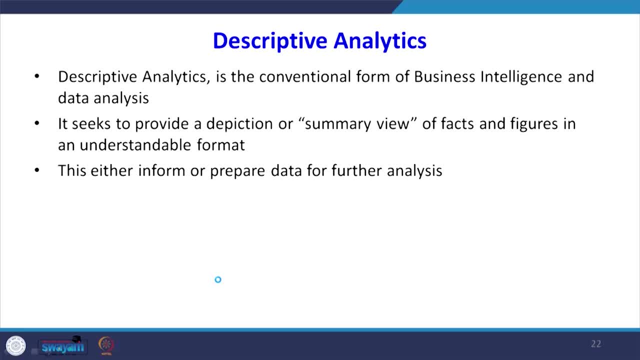 Ok, In an understandable format, This either inform or prepare data for further analysis. So descriptive analysis, or we can say another way in statistics, can summarize raw data and convert it into a form that can be easily understood by humans. They can describe in detail about an event that has occurred in the past. 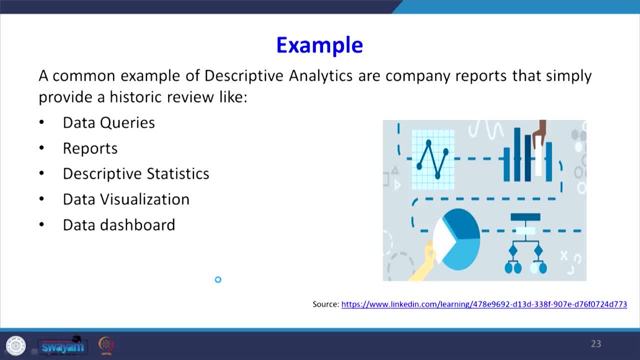 Ok, Some of the examples of descriptive analytics: Descriptive analytics- Descriptive analytics is a common example of descriptive analytics- are company reports that simply provide the historic review, like data queries reports, data descriptive statistics, data visualization and data dashboard. Ok, 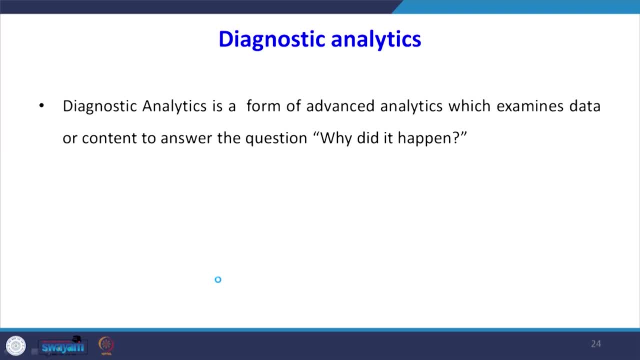 The next one will go to the diagnostic analytics. Diagnostic analytics is a form of advanced analytics which examines data or content. to answer the question: Why did it happen? So we are diagnosing. Suppose we are meeting a doctor for consulting, So he will try to understand why this has happened. 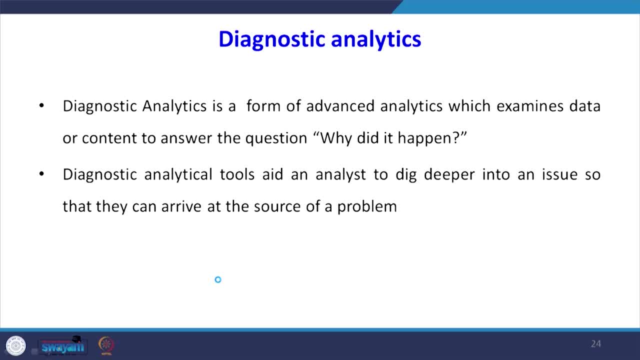 Ok. So that kind of analytics, nothing but diagnostic analytics. So the diagnostic analytical tools aid an analyst to dig deeper into an issue so that they can arrive at the source of the problem. So doctor also will identify if somebody has got some disease. what was the sources of the? 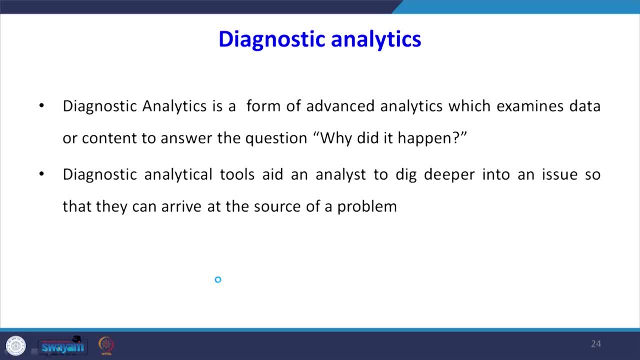 problem. Similarly, the diagnostic analytics also. if something has happened, for example, the company is not performing well, that diagnostic analytics will help you to identify what was the core reason for that. Ok, In a structured business environment, tools for both descriptive and diagnostic analytics go parallel. 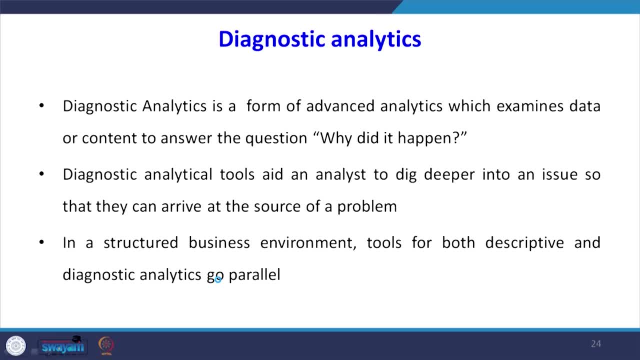 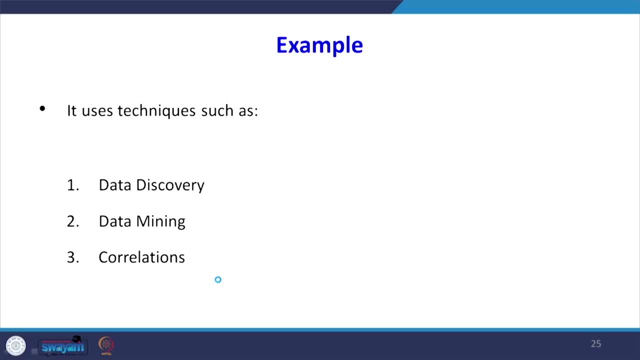 So, when you look at the- whether it is a prescriptive or diagnostic analytics- the tools- analytical tools- which are using- can be same, only the purpose may be different. For example, Data discovery, data mining, correlations. these tools can be used for your prescriptive. 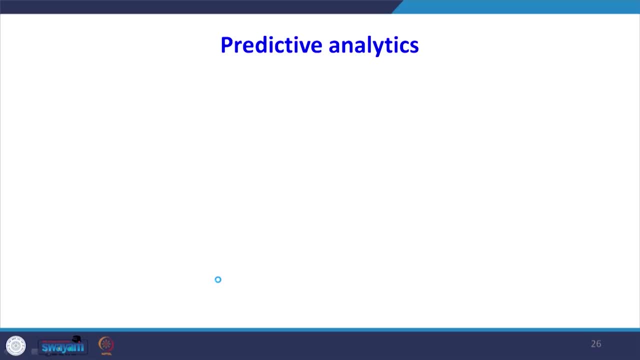 analytics also. Ok, Now we will go for predictive analytics. Predictive analytics helps to forecast trends based on the current events. when you say predicting, obviously it says that it is discussing about what will happen in future. Predicting the probability of an event happening in future are estimating. 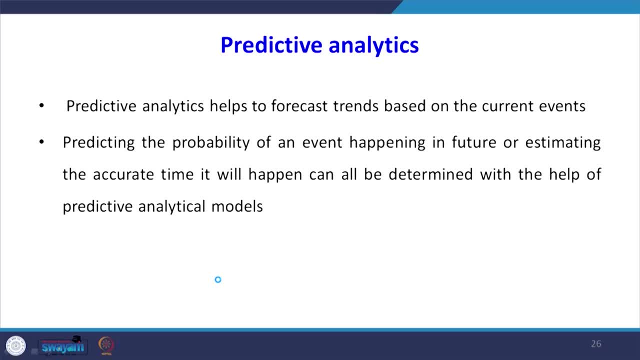 Ok. Accurate time it will happen can all be determined with the help of predictive analytical models. Many different but co-dependent variables are analyzed to predict a trend in this type of analysis. So in the predictive analytics one of the tool is regression analysis. there may be some 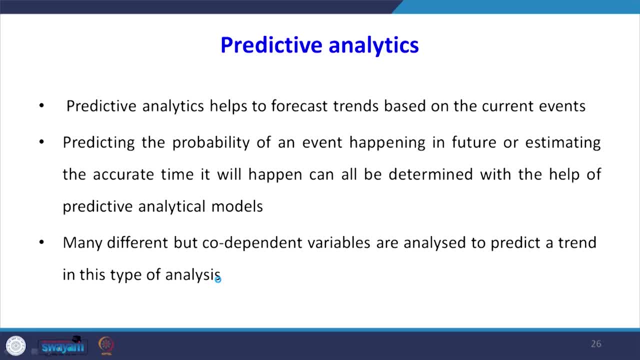 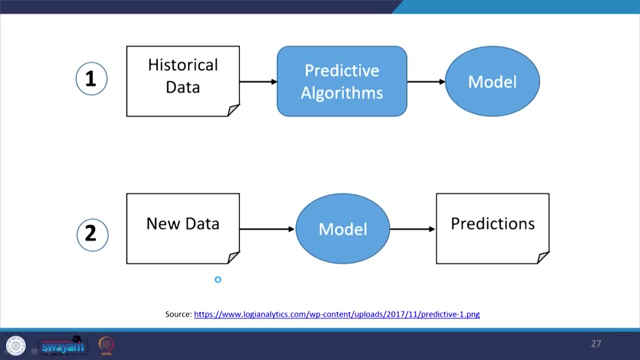 independent variables, some dependent variables, sometimes more dependent variable, more than one dependent variable, and how these variables are interrelated. So that kind of study is nothing but your predictive analysis. Ok, When you look at this picture, you see that, with the help of historical data, by using 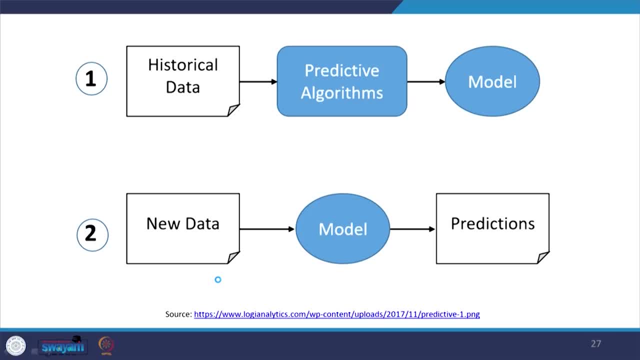 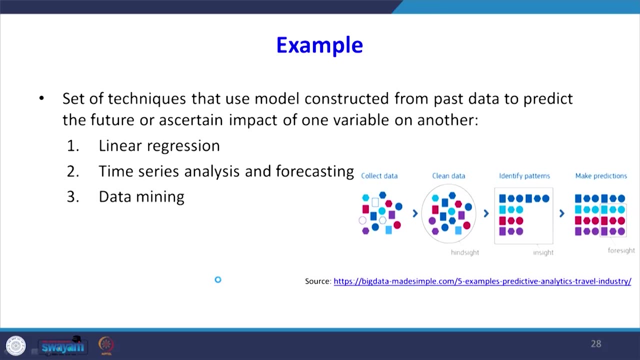 different algorithm- predictive algorithms- you can come with a model. Once the model is developed, a new data can be fit into this model, So we can get some predictions about the past events. Ok, Example is linear regression: time series analysis and forecasting linear regression. 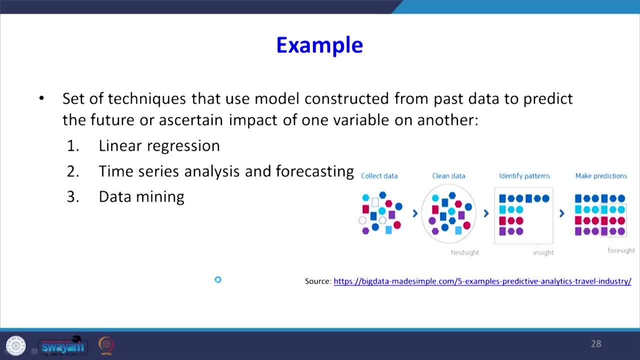 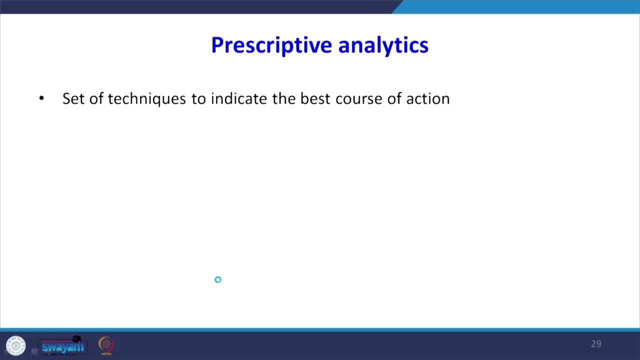 data mining. These are the techniques for predictive analytics. The last one is a prescriptive analytics, a set of techniques to indicate the best course of action. It tells what decision to make to optimize the outcome. The goal of prescriptive analytics is to enable quality improvements, service enhancements. 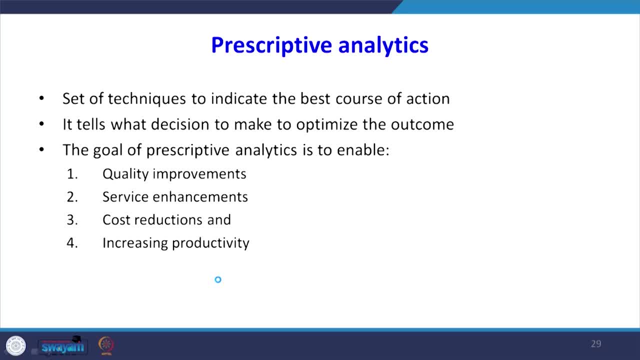 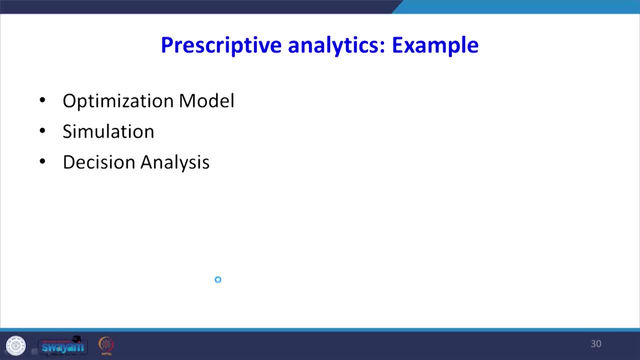 cost reductions. The curve net line is designed towards Jeremy Halperin's math model point of influence, Theужin and increase in productivity. ok, In the prescriptive analytics some of the tools which we can use as optimization models, simulation model, decision analysis. these are the tools under prescriptive analytics. 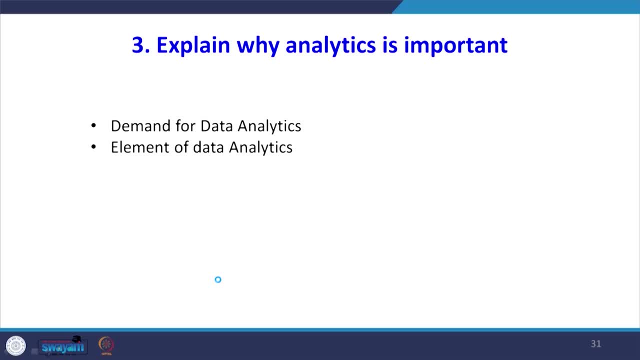 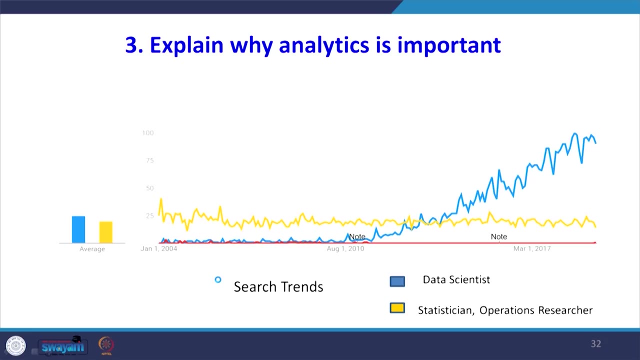 Next is we are going to see why the analytics so important. In this section we will see what is happening. that demand for data analytics, MATCH connections. we look at the different elements of data analytics. This picture shows Google trends. This was up to 2017.. See, for example: the blue represents the data scientist, this orange- 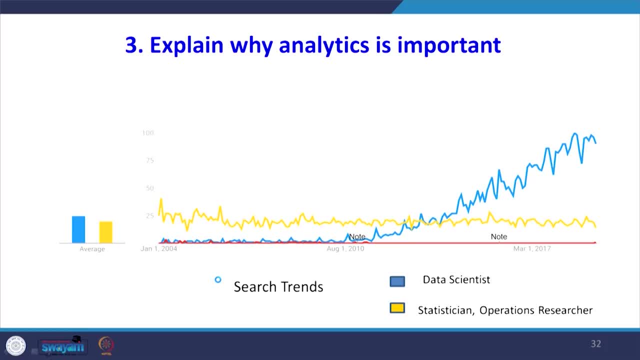 represents the statistician operation researchers. You see, the trend is it is increasing. that means people are searching in the Google search engine the word data scientist more number of times. See the. the search count is it is increasing that means there is a demand for that particular say job. You see, if you look at this, this is the newspaper. 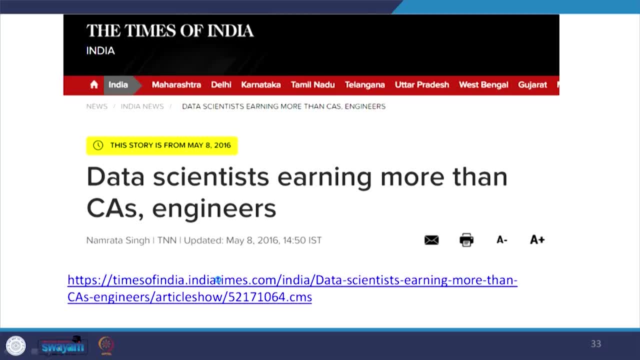 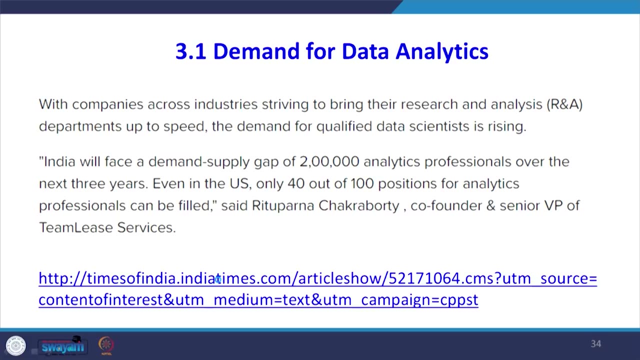 clipping from Times of India. There are so many news are coming about data scientist and the future requirement of data scientist. You see the data scientist earning more than more CAs and engineers. you can look at this link for further and you see the demand for. 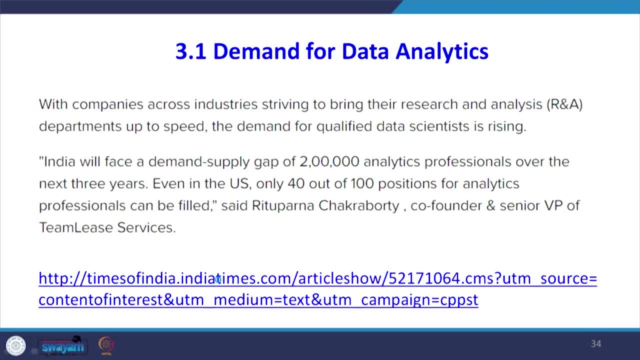 data analytics. This is also newspaper clipping, With companies across industries striving to bring their search and analysis department up to speed. demand for qualified data scientist is rising, So there is an emerging field. So many companies is looking for the qualified data scientist. So if you take this course, 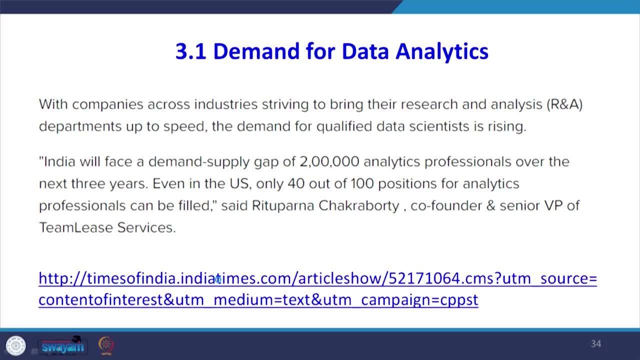 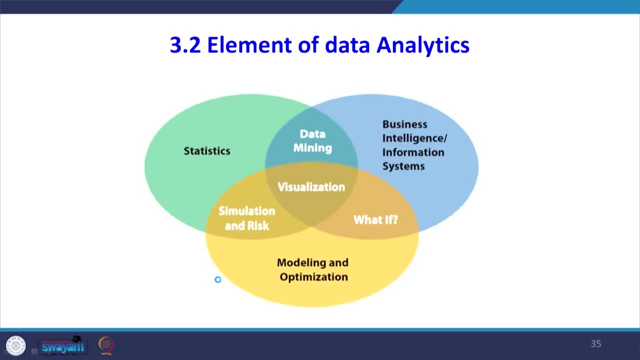 it is very difficult at end of the course that you may be qualified for getting into this companies. Many time you see what is data analytics, statistics, data mining, optimizations. these are students having different understanding on that. So when we say data analytics, there are different element. one is statistics, next one is the 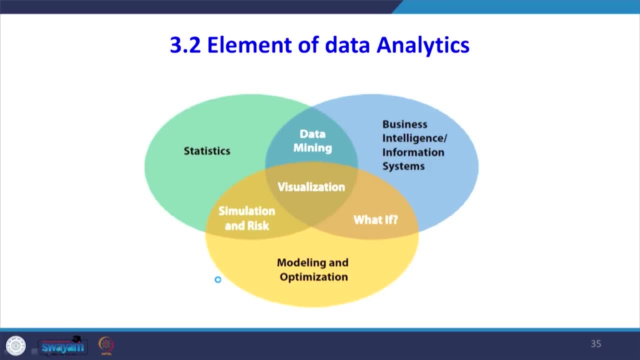 business intelligence information systems, then modeling and optimizations, then simulation and risk. we can say: if you are able to do what-if analysis. that is nothing but sensitivity analysis, visualization, data mining- these are the components of data analytics and how these different domains are interrelated. 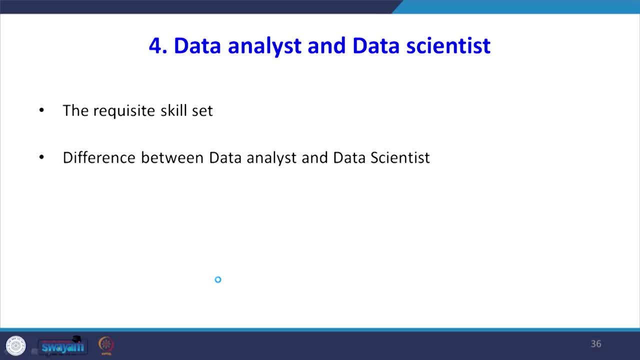 Next we will see what kind of skill set is required to become a data analyst. then we will see the small difference between data analyst and data scientist. Okay, See, to become a data analyst is the basic, fundamental knowledge. is you need to have knowledge of mathematics? 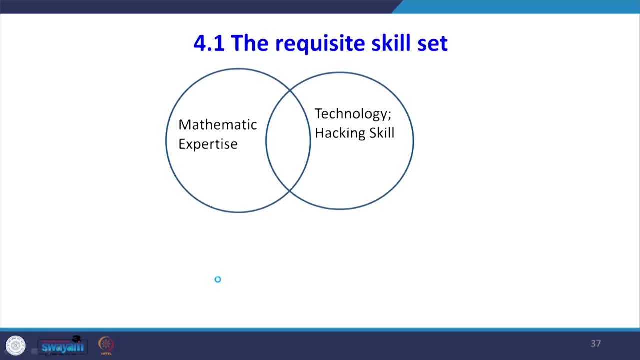 Next you need to have the knowledge of technology is nothing but hacking skill. Hacking skill is the sense if the data is given, hacking is done in the look at the positive way, how to use the data to get more informations. The next skill is business and strategy acumen. 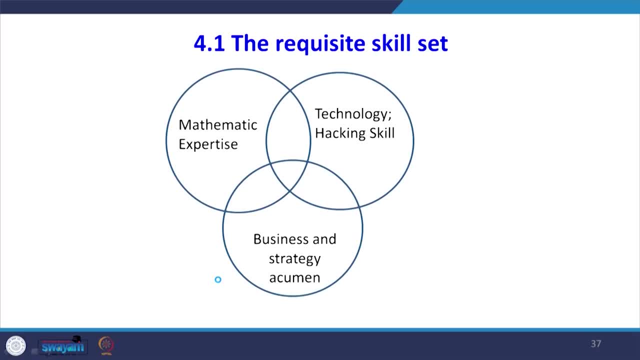 You should have the knowledge of the domain, knowledge of the business, and you need to have the strategy acumen. So these three skills are required for a good data scientist. It is very difficult to have a one person will have all these three skills. that is why 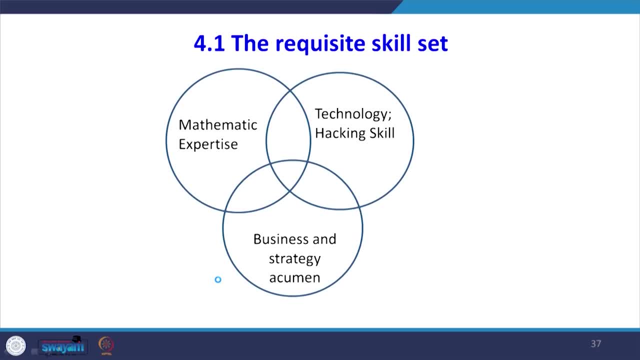 availability of good data analytics is becoming very difficult, because somebody may be very good at mathematics, but they may not have very good knowledge and business. Some people may have very good technology. they may not technology in the sense, information technology. they may not have good knowledge on the business knowledge, or, and so on. 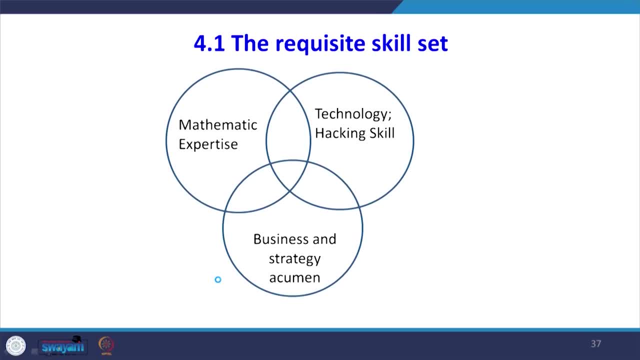 So we need to have the combination of all these three skills, otherwise the group of people- some people from mathematics department, mathematics area, some people from computer science, some people from the domain knowledge- they have to work together to form a good data scientist team. 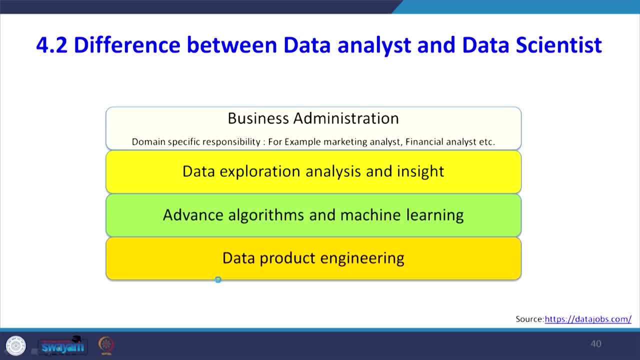 Okay, This forms data science. Now, what is the difference between data analyst and data scientist? and the difference is what kind of role they are doing. For example, the role of a data analyst is: see in a business context. he may have the knowledge of business domain, for example, if he is good at doing analytics in the area. 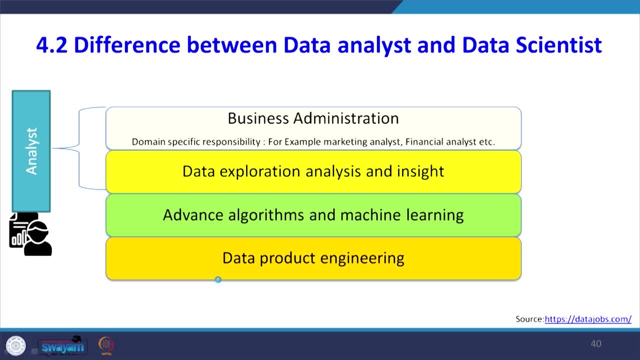 of marketing, he can be called as a marketing analyst. If the person is from finance area, he can be called it is a finance analyst. So he is the analyst, data analyst, But the role of data scientist is little bigger, because the data scientist need to have the 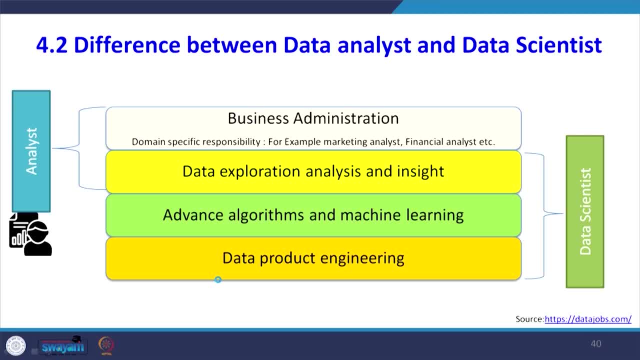 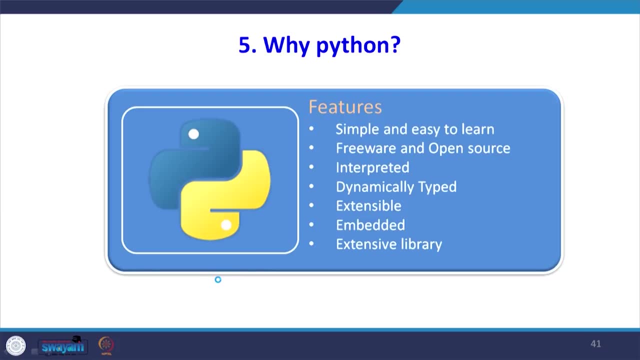 knowledge of advanced algorithms and machine learning and able to come out with a data product, which I told you in the previously. So the data scientist can come out with a data product. Okay, In this course we are going to use Python In this. in the next lecture I will tell you the basic introduction about the Python. 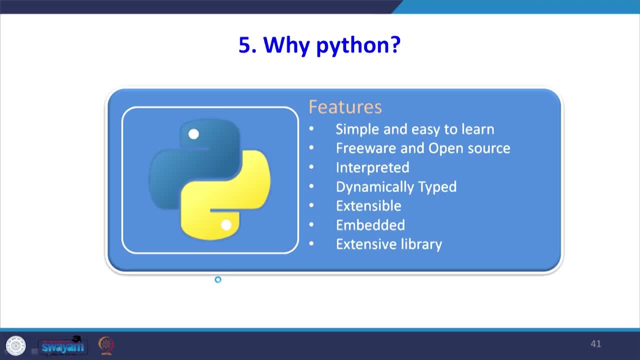 Here we will see why we are going to use the Python, Because Python is very simple and easy to learn. Most importantly, it is a freeware and open source. It uses interpreted. it is not the compiler, suppose. what do you mean by compiler and interpreter? 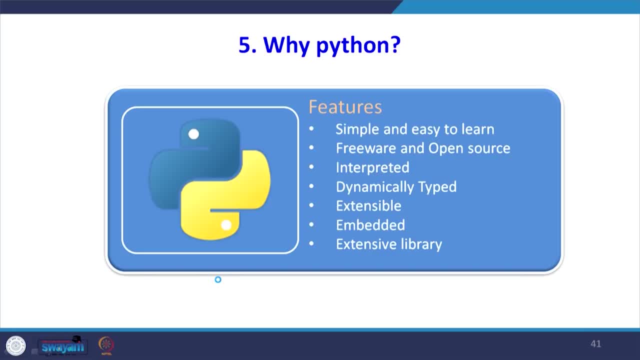 is You need a compiler to solve the whole program, But interpreter need not be. in that way it can solve even you can interpret one sentence also, one line in the programming line also. It is dynamically typed, dynamically typed to the sense in some other programs every. 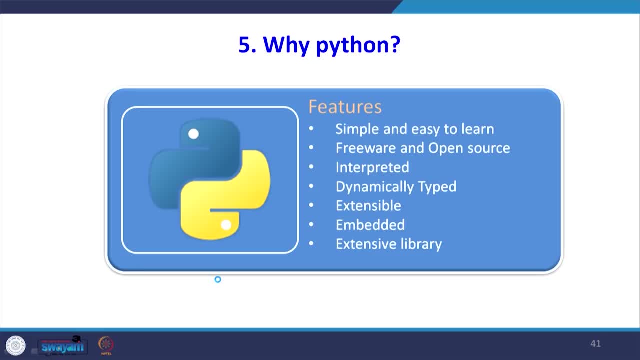 time you have to declare the variable. what is the nature of the variable, whether it is integer, whether it is a float. But here you need not do. it is dynamically, it takes the value. It is extensible, extensible sense. Okay, So if you make a code in some other language that can be extended with the help of Python, 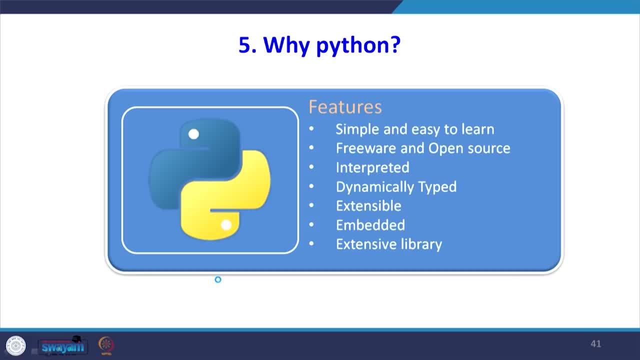 and can be embedded- embedded in the sense you have made some program in Python. It can be embedded with some other platforms and it has extensive library. The usability of Python is it is a desktop and web applications. It can be used for data applications. 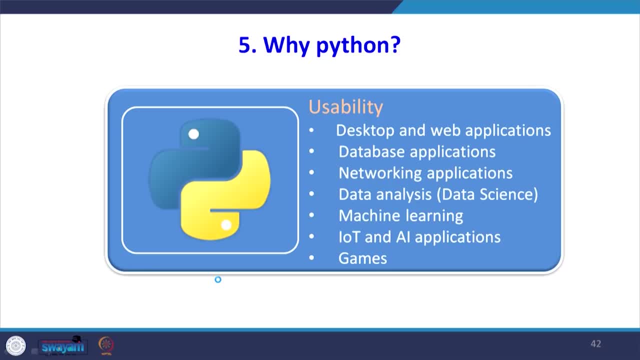 It can be used for networking applications. Most importantly, it can be used for data analyst, data science. Okay, It can be used for machine learning. It can be used for IoT- Internet of Things and artificial intelligence applications, and can be used for games. 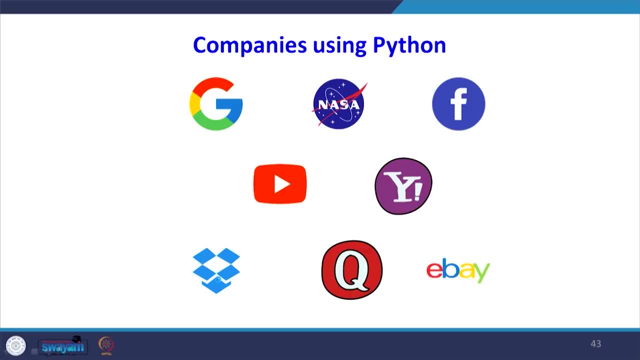 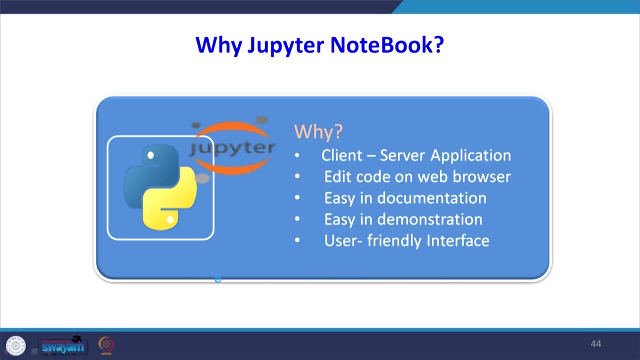 The another reason for choosing Python is most of the companies they use Python as a language in their in their company, like, for example, Google, Facebook, NASA, Yahoo and so eBay. they use Python as a programming language In this Python also, we are going to use a Jupyter notebook. in the next class. I will explain. 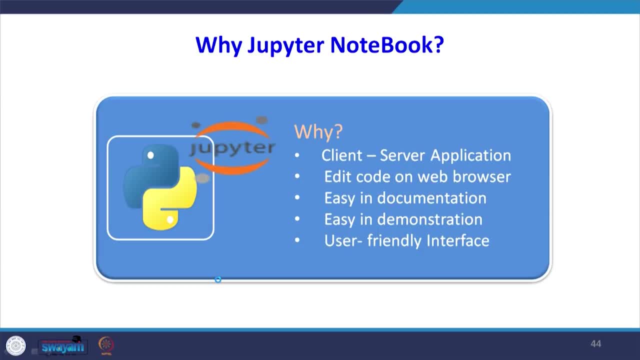 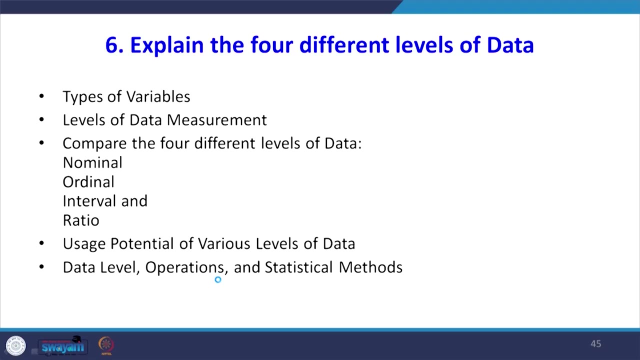 it Because it is theclient server application is edit code on web browser, easy in documentation, easy in demonstration and user friendly interface. This was the last session of the this lecture. we will explain four differentlevel of the data. One is the type of variables. level of data of measurement. compare four different level. 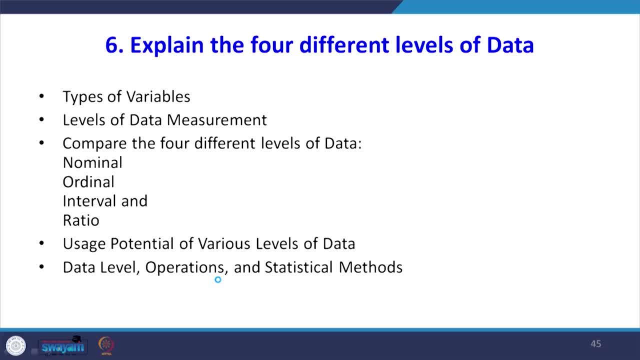 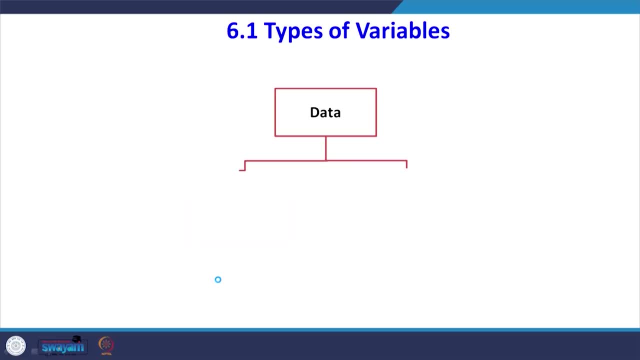 of data will say nominal, ordinal interval and ratio. Okay, We see that. why what is the usage of knowing this different level of data? The one way for classifying the data is the categorical data. one is a numerical data. In categorical data you see marital status, political party, eye color. these are categorical. 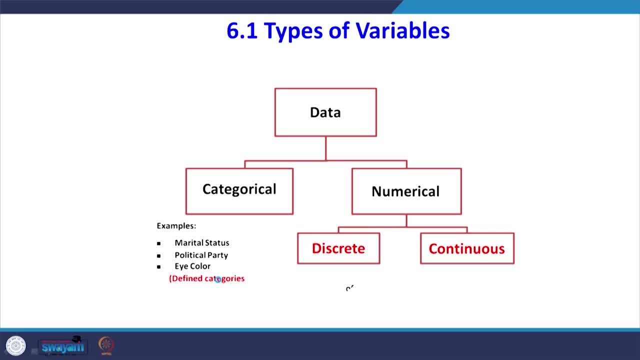 data, Numerical data. it can be discrete or continuous. Discrete data may be a number of children, defects per hour, so it is the discrete data, Okay. Continuous data may be weight voltage. these are the example of continuous data. So what is the difference between discrete and continuous? is, you say, a number of children? 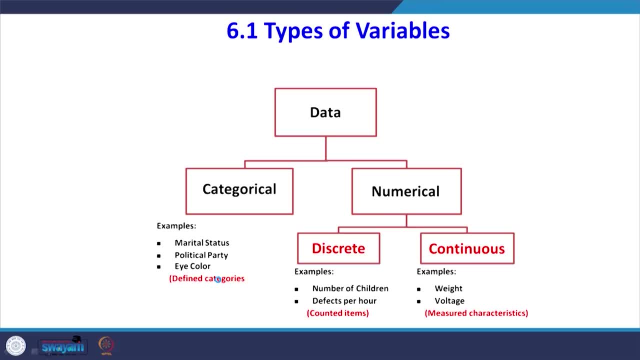 you may say 2 children or 3 children, 2.5 children is not possible. But in continuous, if you look at between 0 and 1, the numbers are continuous. there is infinite number of values are there between 0 and 1, so it is a continuous variable. 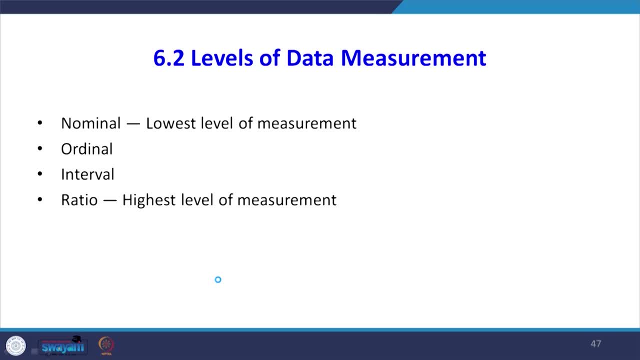 Next we will see the different levels. So what is the difference between discrete and continuous? So what is the different level of data measurement? previously we have seen the classification of data. we classified as the categorical data, numerical data. There is another way of classification is classifying it: nominal data, ordinal data, interval data. 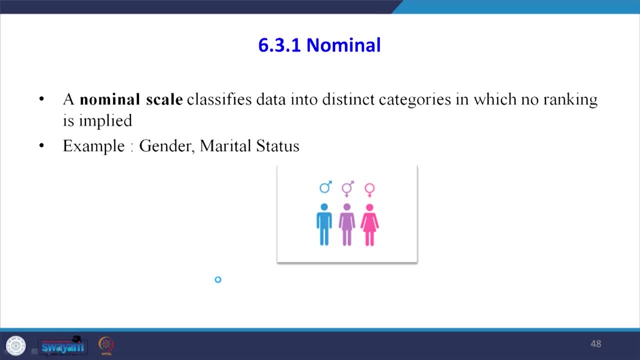 ratio data. We will look at the. what is a nominal data? Nominal scale scale classifies data into distinct categories in which no ranking is implied. The example of nominal data is gender, marital status: Okay, Marital status, for example, gender. suppose you are conducting a questionnaire. suppose 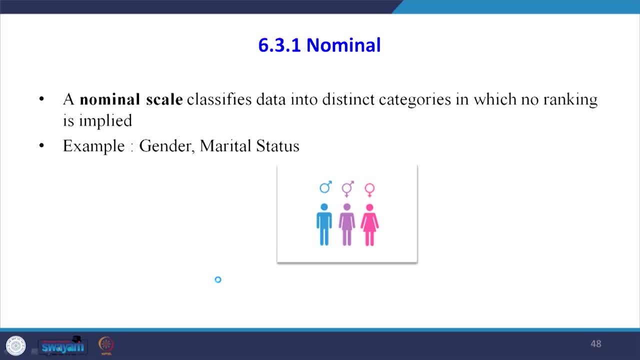 you have captured the gender: male 0, female 1. this 0, 1 represents just the gender. You cannot do any arithmetic operations with the help of the 0 and 1, for example. you cannot find out the average. software will give you some number, but there is no meaning for that. 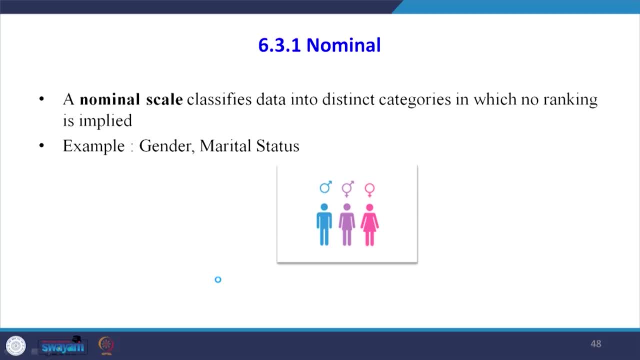 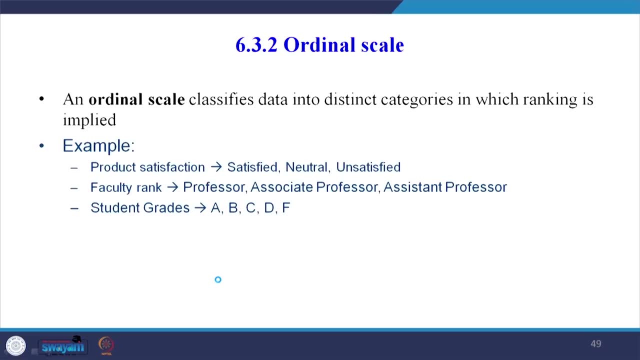 Similarly, marital status, whether it is married, Marital status- Marital status- Marital status- Unmarried. This is the example of nominal data. The next level of data is the ordinal scale. it classifies data into distinct categories in which the ranking is implied. 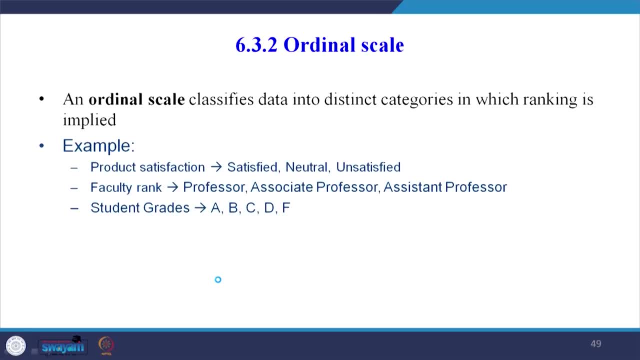 Here the numbers are the ranked. for example, you may ask the customer to give you a ranking about the their level of satisfaction, for example, satisfied, neutral, unsatisfied. Okay, The faculty ranking- professor, associate professor, assistant professor. you see that their rank is followed. 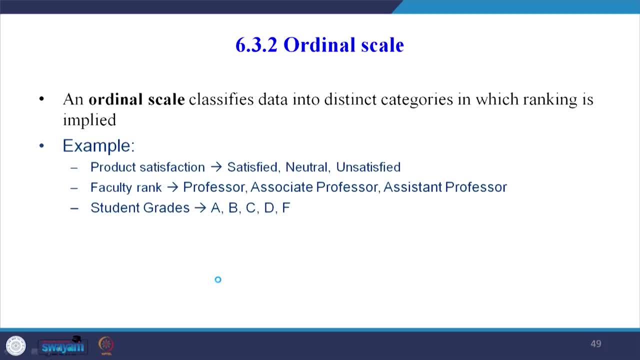 For example: 1 professor, 2 associate professor, 3 assistant professor, Student grades A, B, C, D, F. these are ranking, because the numbers 1,, 2, 3 represent the rank. The next level of data is interval scale. 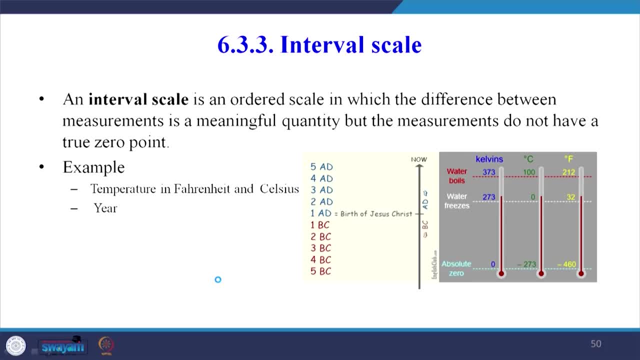 The interval scale is ordered scale in which the difference between measurement is a meaningful quantity but the measurement do not have true zero point. The example of interval scale is, for example, year. say now, say this year is 2019, you can add and subtract something. 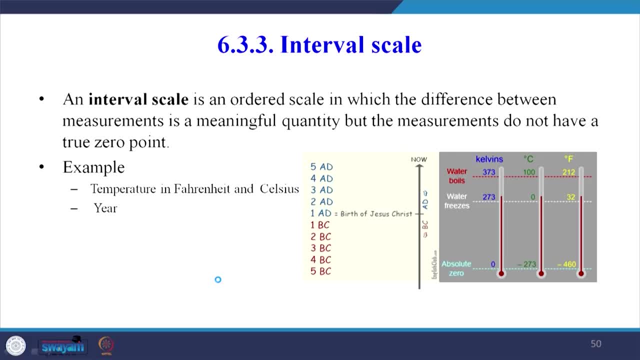 You can add another 5 years- 2024- or you can subtract another 9 years- 2010,. but you cannot multiply. If you multiply that number- for example, 2019 and 2020, you will end up with a big number. there is no meaning for that. 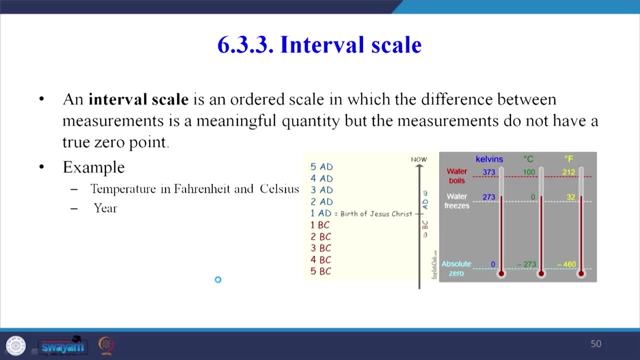 Because there is no meaning for zero. The another example of interval scale is your Fahrenheit temperature, For example. in the Fahrenheit scale the zero represents freezing point, but it is not the absence of the seat but absence of the temperature. But the same time in the kelvin, for example, minus 273, it is absence of heat, so kelvin. 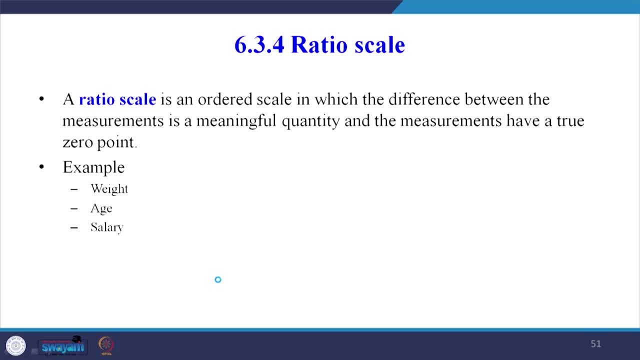 will be the some other scale that you will see. the next one Scale is the ordered scale in which the difference between the measurement is a meaningful quantity and the measurement have the true zero point: weight, age, salary and the Kelvin temperature. 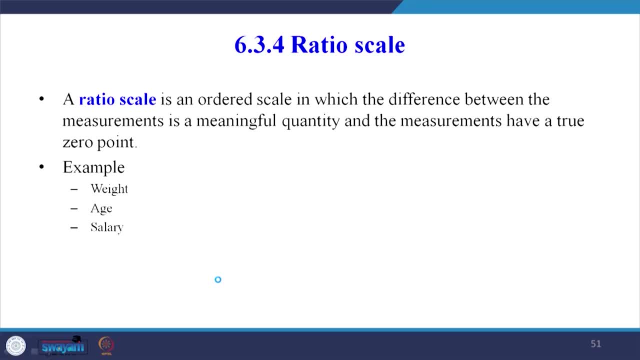 comes under ratio scale, because 0 Kelvin that means the absence of the heat. So the ratio scale. you can do all kind of arithmetic operation, for example the nominal. you cannot do any arithmetic operation in ordinal. you cannot do any arithmetic operation in the interval. you can add and subtract, but you cannot multiply. but in the ratio. 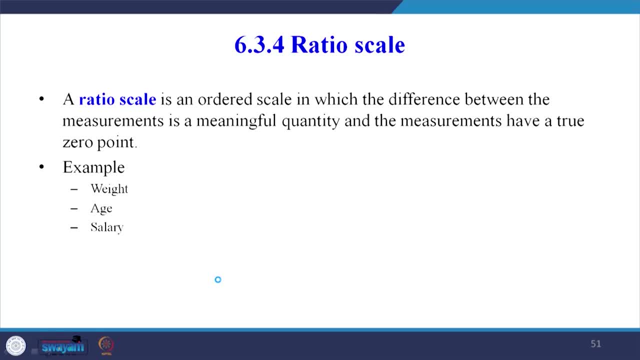 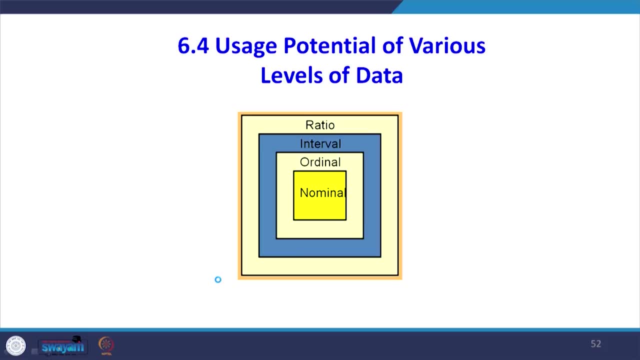 data. you can do all kind of arithmetic operation. you can add, you can subtract, you can multiply, you can divide. You see the usage potential, various level of data. for example, the usage potential of nominal data is not that much. the next one is ordinal, next one is interval, next one 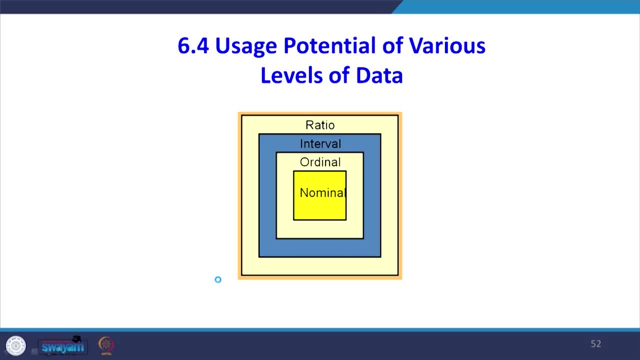 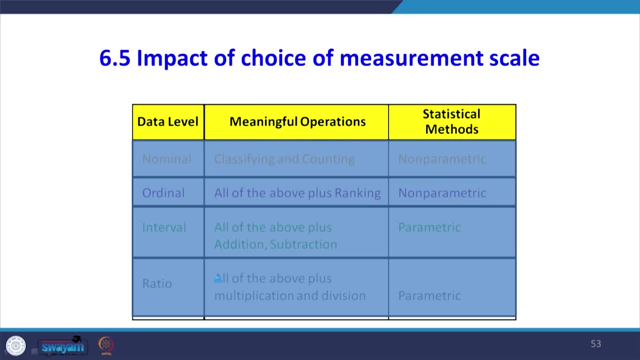 ratio. So the ratio data is having the highest value, The highest usage potential. the nominal data is having the least usage potential. This is more important why we have to know the different types of data, because this types of data is helping to choose the right analytical tools for doing analysis. 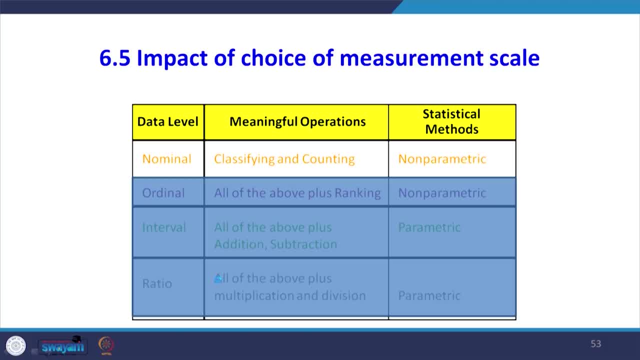 For example, the data is the nominal data, you can do only non-parametric test. For example, For example, if the data is ordinal, here also you can do only non-parametric test. But if the data is interval you can do parametric test. 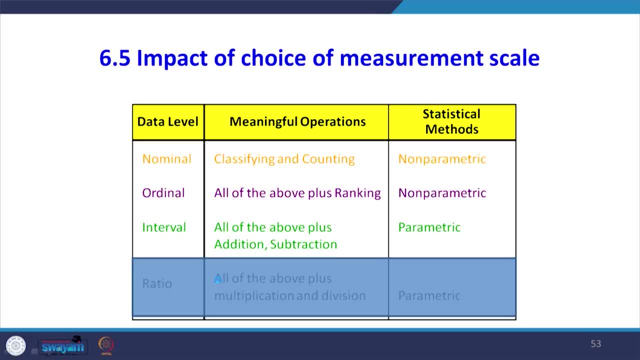 You see that intervalyou can do all of the above, plus addition and subtraction In the ratio. you can do all of the above, plus multiplication and division. Ok, And statistical methods. you can go for parametric methods. So the purpose of classifying the data into nominal ordinal interval ratio is to choose. 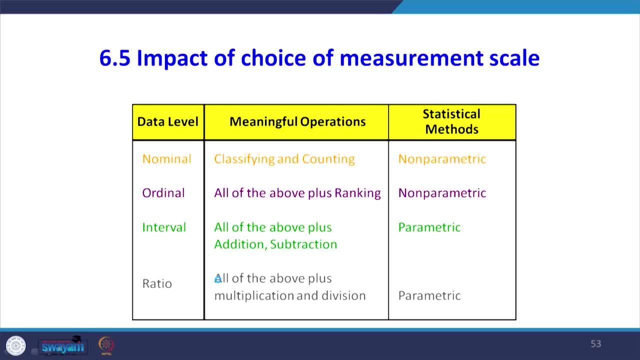 the right analytical tools, whether it whether it is a parametric or non-parametric. The other reason is sometime, for if we want to do a non-parametric analysis that is used only for nominal data, Sometime the students they will. the data may be nominal but they may go for a parametric.